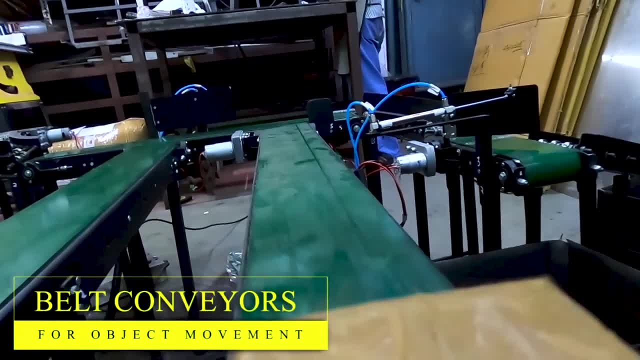 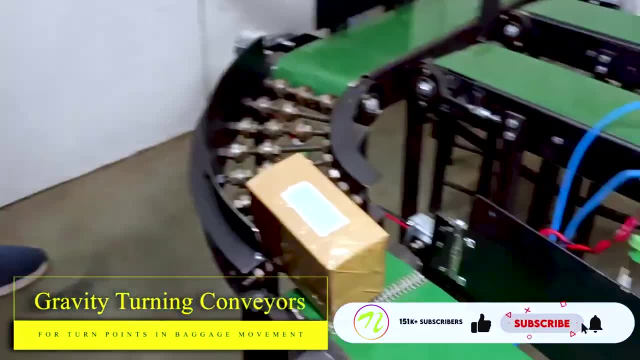 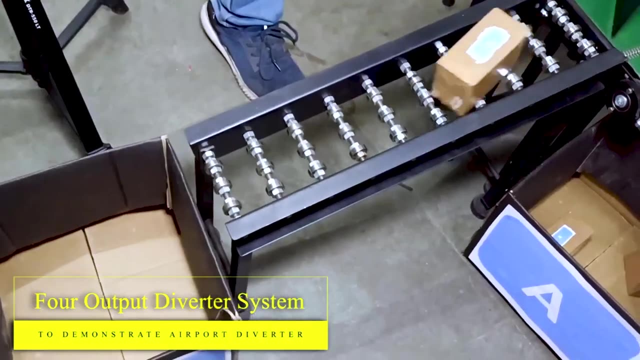 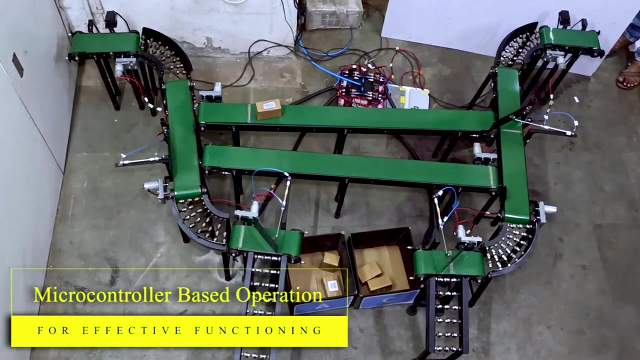 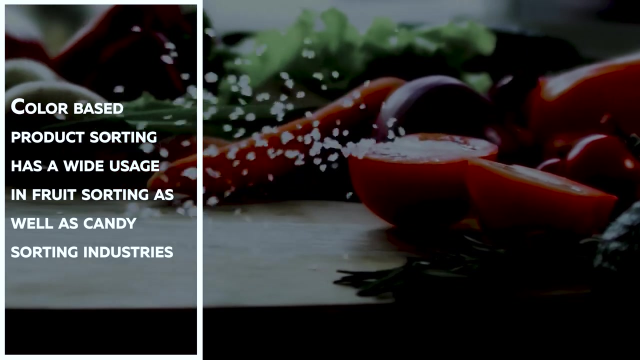 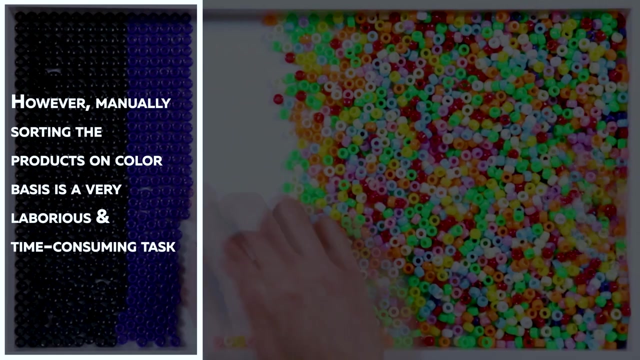 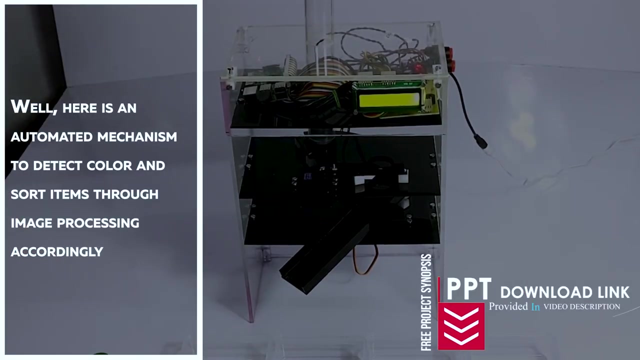 eens on the Oh Color Based Product Sorting. Color based product sorting has a wide usage in fruit sorting as well as candy sorting industries. However, manually sorting the products on color basis is a very laborious and time consuming task. Well, here is an automated mechanism to detect color and sort items through image processing. 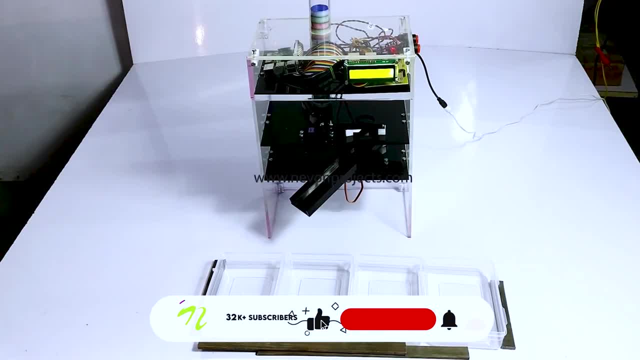 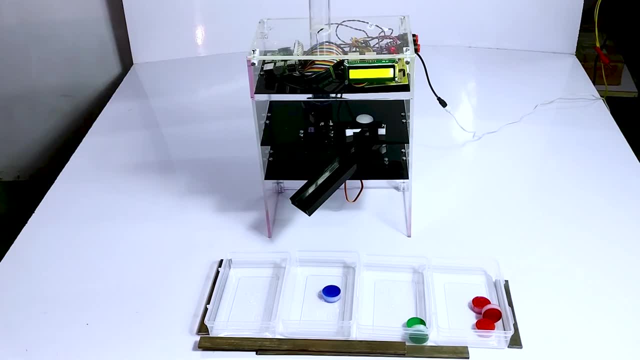 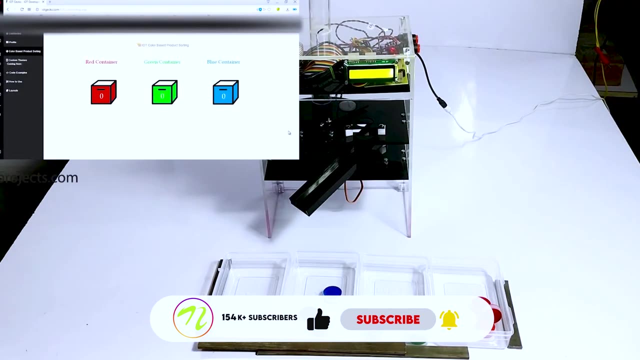 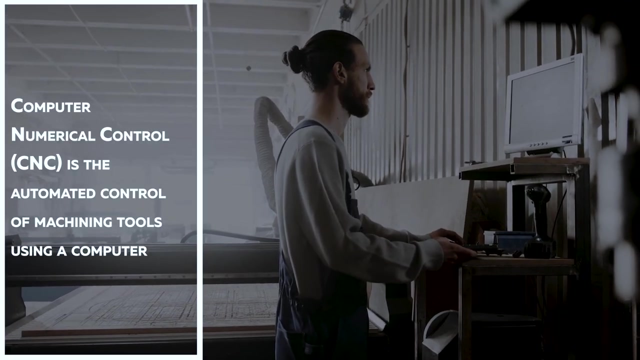 accordingly, 3-axis CNC Machine. Computer Numerical Control is a machine that is used to process the color of a particular item. It is used to process the color of a particular item. Well, here is an automated mechanism to detect color and sort items through image processing. 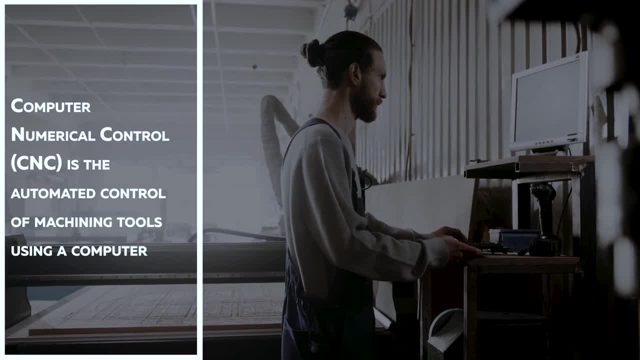 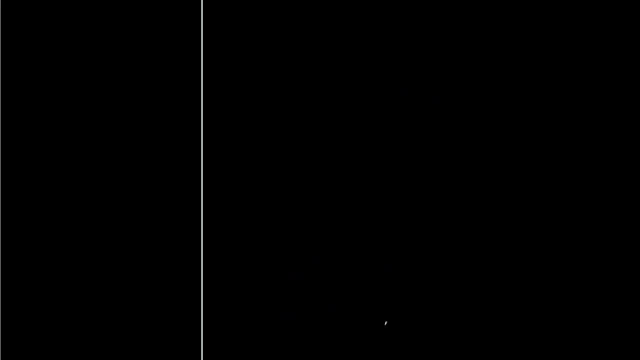 accordingly. Here is an automated mechanism to detect color and sort items through image processing. It is the automated controls of machining tools using a computer. Along with reducing the human effort required, CNC machines also boost accuracy and precision. This 3-axis CNC machine uses an array of stepper motors for engraving and cutting. 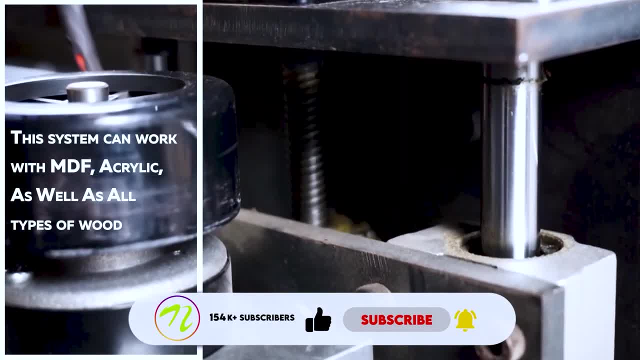 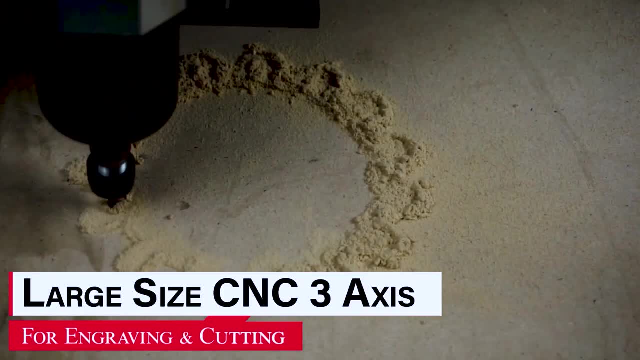 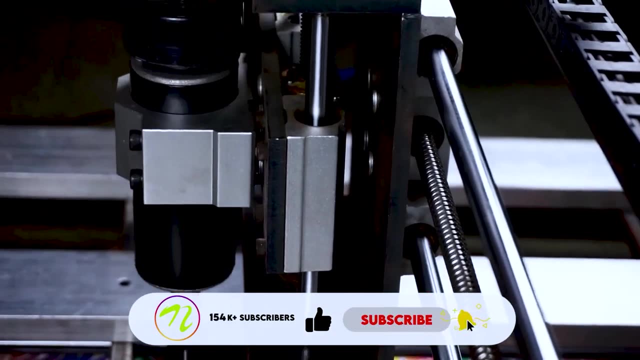 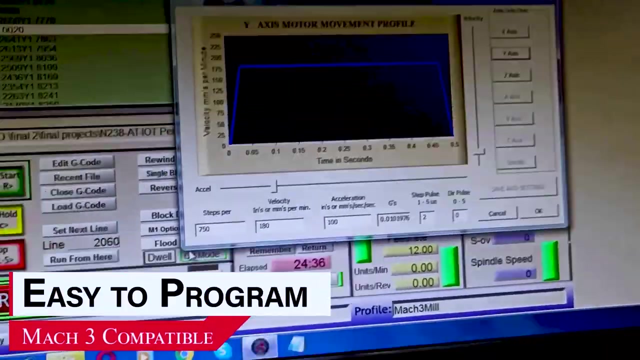 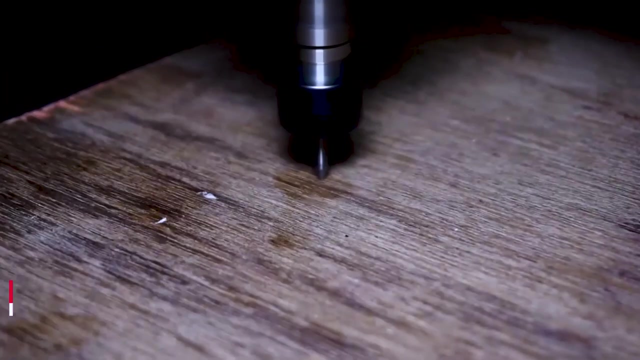 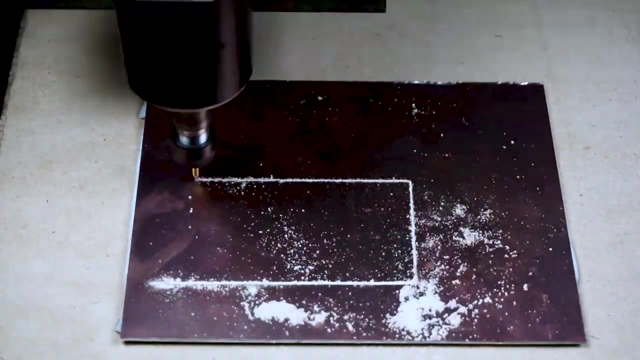 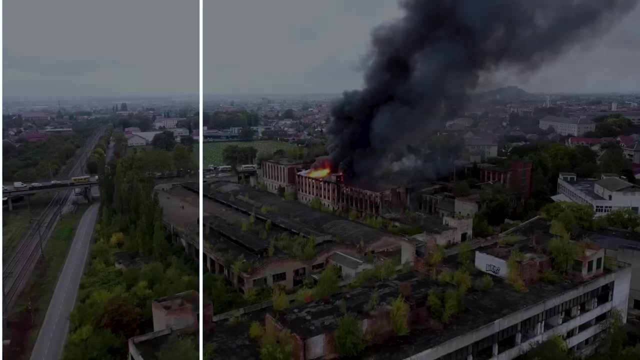 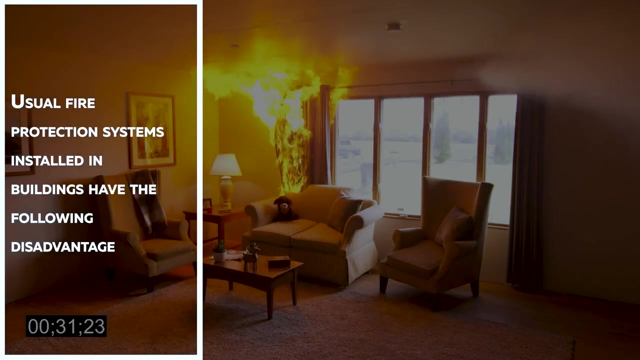 The system can work with MDF, acrylic as well as all types of wood. Money rotating fire protection system. Large industrial and commercial facilities always run the risk of a fire breaking out. Usual fire protection systems installed in buildings have the following disadvantage: They spray small. 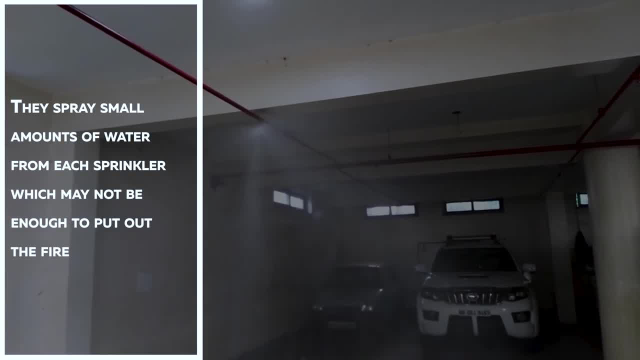 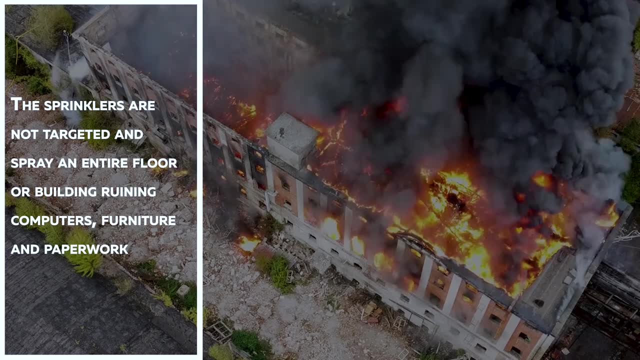 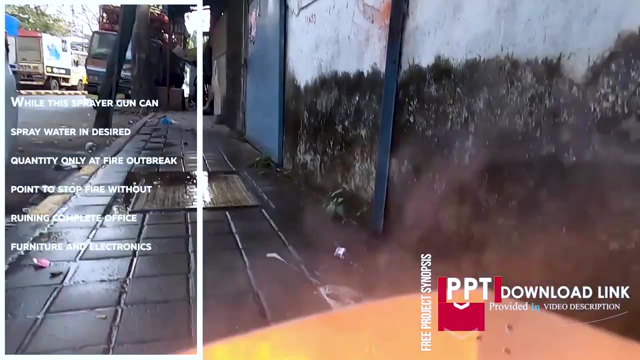 amounts of water from each sprinkler, which may not be enough to put out the fire. The sprinklers are not targeted and spray an entire floor or building, ruining computers and furniture and paperwork of the entire building, While this sprayer gun can spray water in desired quantity only at the fire. 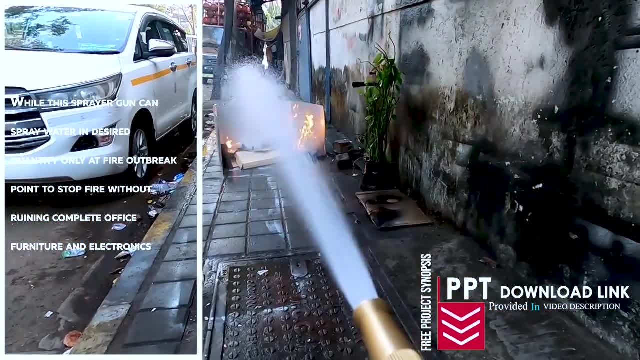 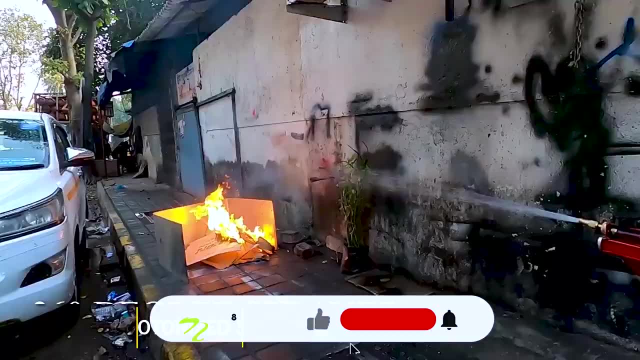 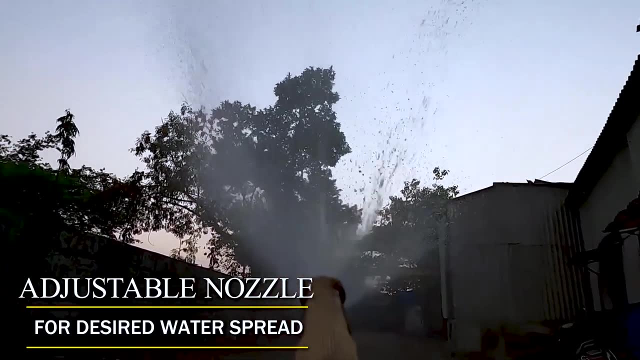 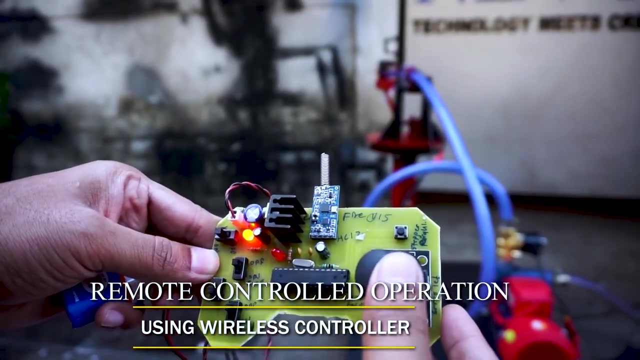 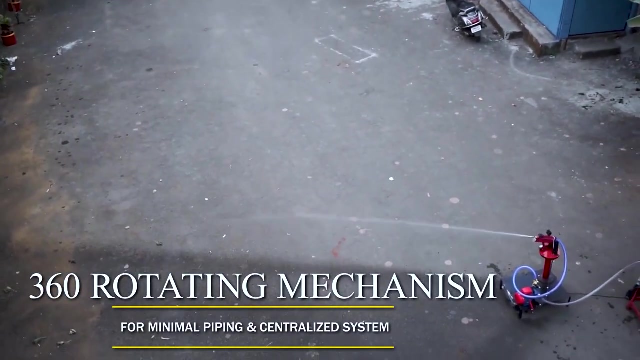 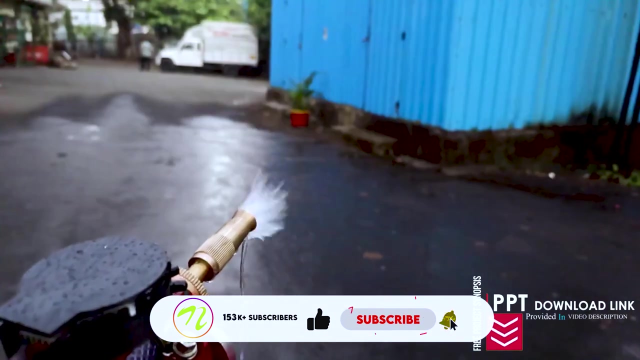 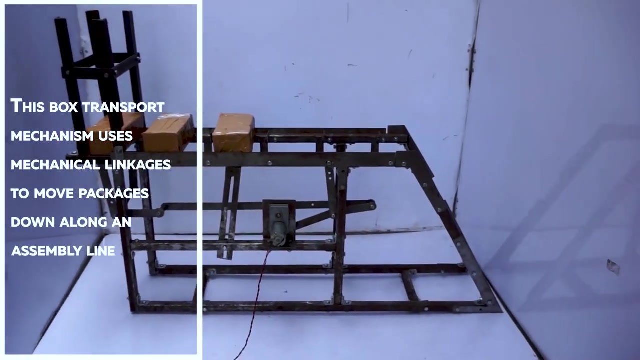 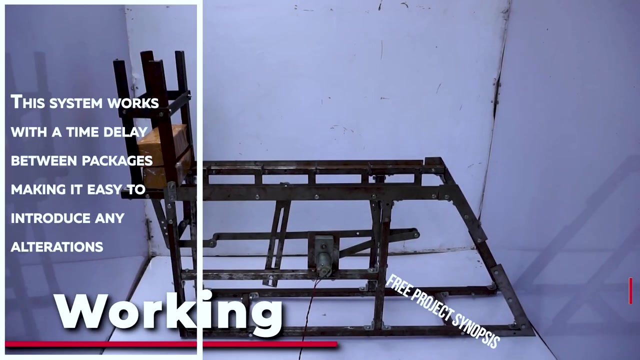 breakout point to stop the fire without ruining the complete office furniture and electronics. Box Transport Mechanism. This box transport mechanism uses mechanical linkages to move packages down along an assembly line. This system works with a time delay between packages, making it easy to introduce any alterations. 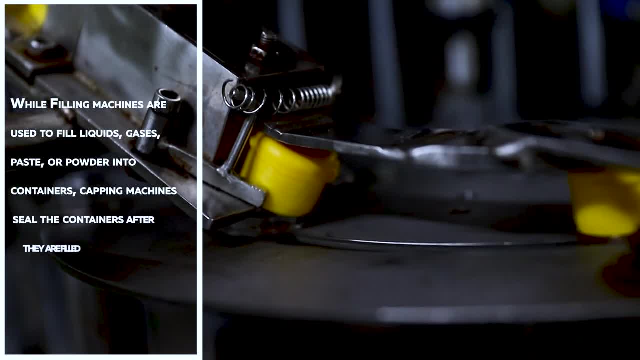 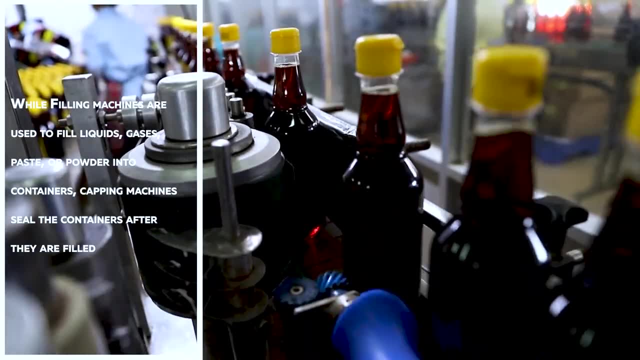 Automatic bottle filling and capping machine. While filling machines are used to fill liquids, gases, paste or powder into containers, capping machines seal the containers after they are filled. Using PLC, this automatic bottle filling and capping machine integrates both these processes into one. 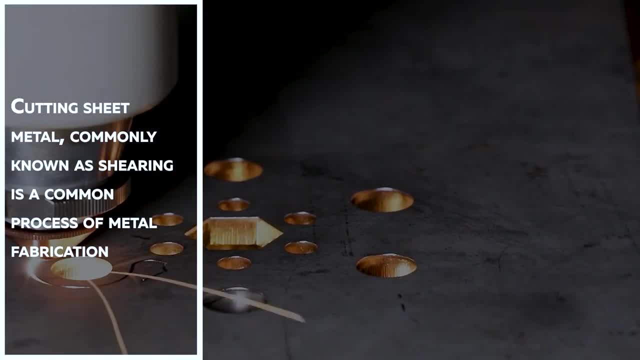 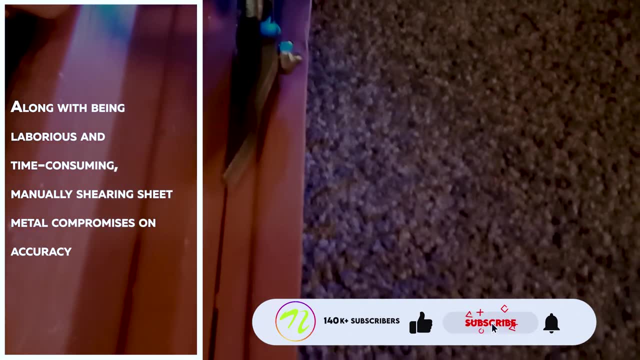 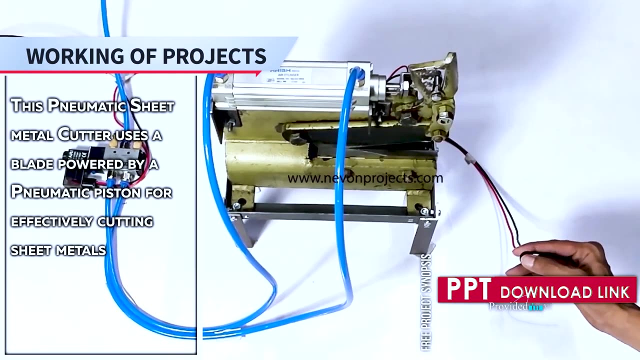 Pneumatic sheet metal cutter. Cutting sheet metal, commonly known as shearing, is a common process of metal fabrication. Along with being laborious and time-consuming, manual shearing of sheet metal compromises on accuracy. This pneumatic sheet metal cutter uses a blade powered by a pneumatic piston for effectively cutting sheet metals. 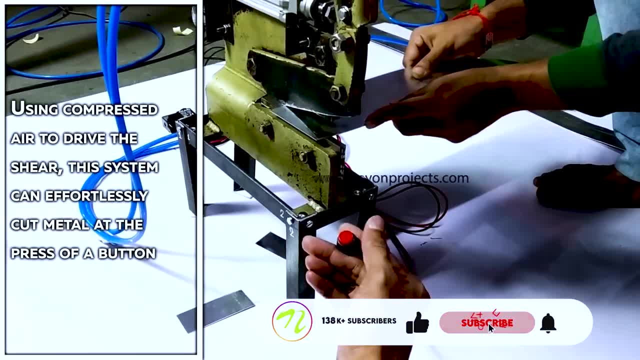 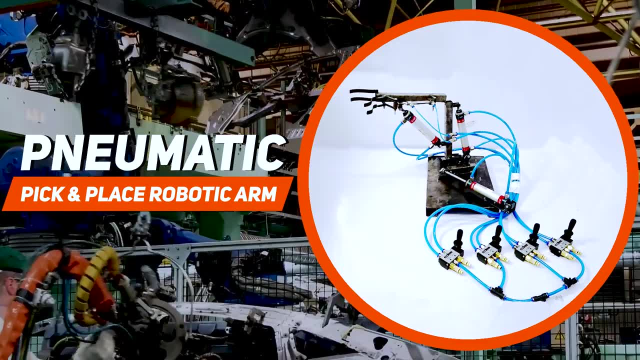 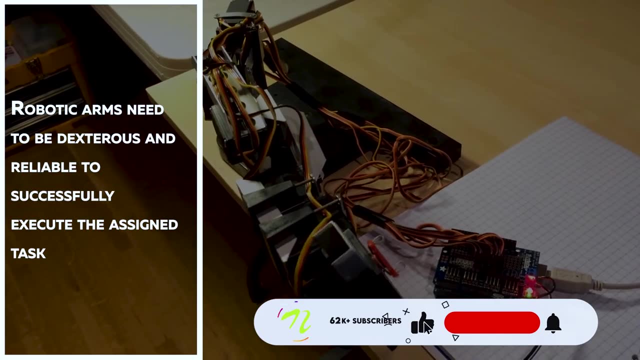 Using compressed air to drive the shear. this system can effortlessly cut metal at the press of a button. Pneumatic pick and place robotic arm. Robotic arms have a broad range of applications in industrial automation. Robotic arms need to be dexterous and reliable to successfully execute the assigned task. 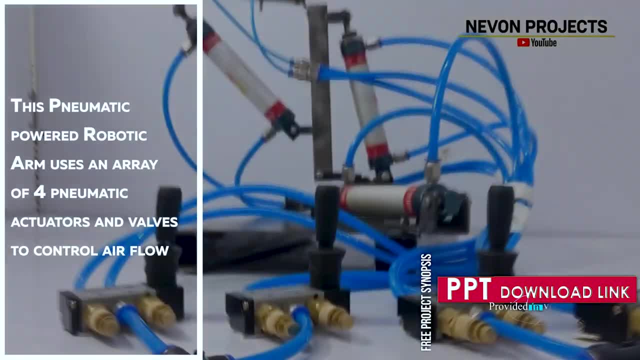 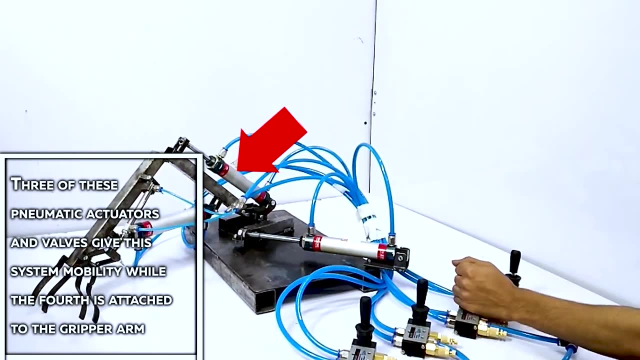 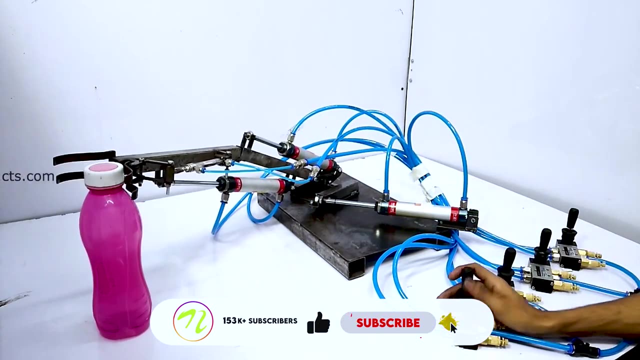 This pneumatic powered arm uses an array of four pneumatic actuators and valves to control the airflow. Three of these pneumatic actuators and valves give the system mobility, while the fourth is attached to the gripper arm. The pneumatic arm uses a fixed spring, with the spring moving forward. 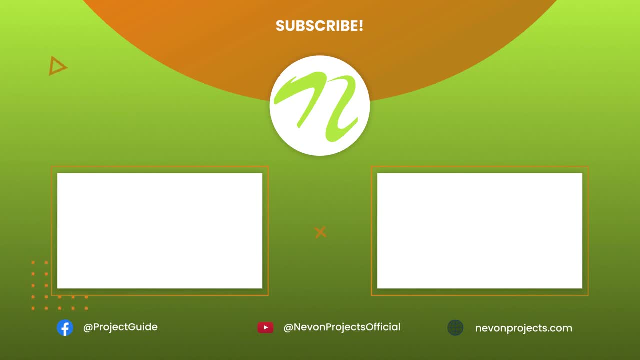 The pneumatic arm is the most powerful and effective way to use the system. Pneumatic pressure sensor at the back of the system is the most effective way to control the airflow.